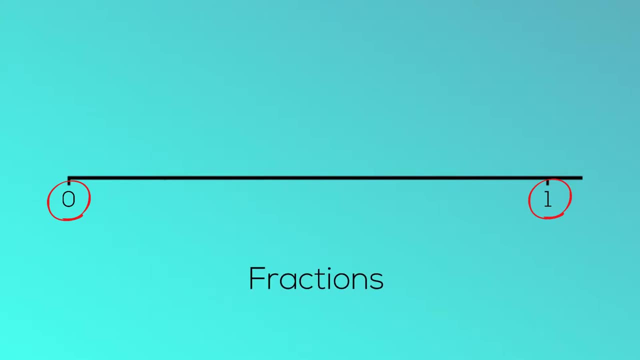 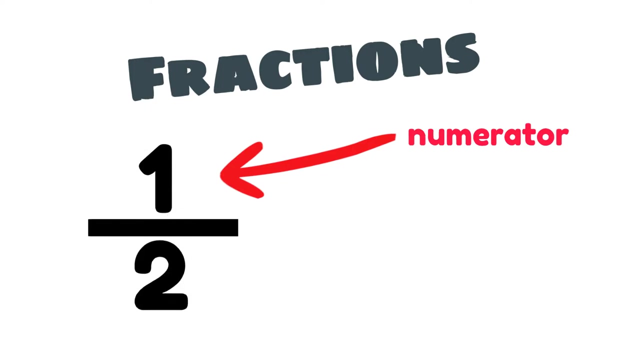 but we can use this space to represent fractions. Before we start finding fractions on number lines, let's review a few important points about fractions. A fraction has a numerator and a denominator. The denominator tells us how many equal parts the whole has been divided into. The denominator in 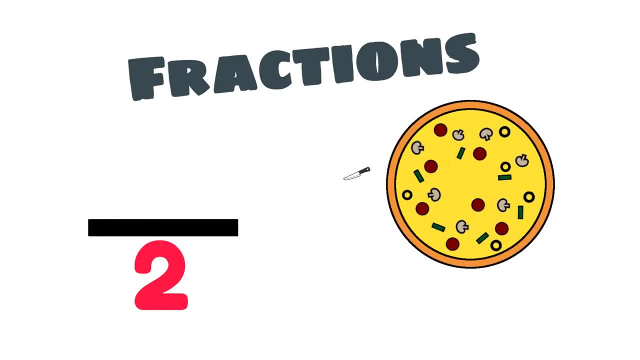 this fraction is 2, so it tells us that a whole has been divided into two equal parts. The numerator tells us how many of these parts we have In this fraction. the numerator is telling us we have one of these equal parts. The fraction is one half. 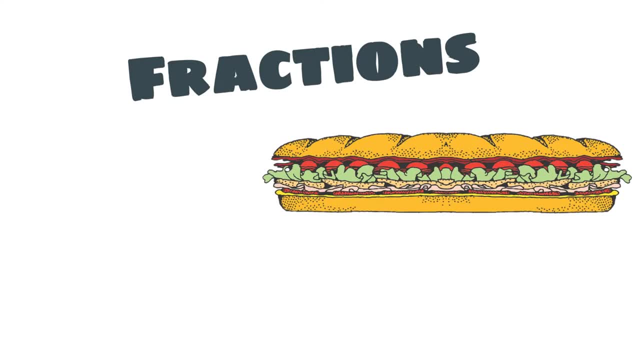 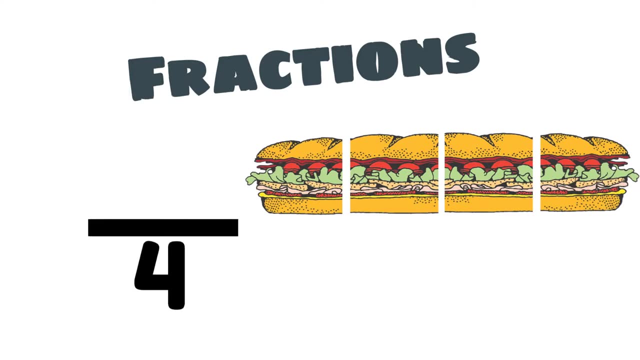 Let's look at another example. Here we have a sandwich that has been cut into four equal parts. That means the denominator will be four. Each one of the equal parts is one fraction. Each one of the equal parts is one quarter. If someone were to be given three of those parts, they would have three quarters of the whole sandwich. 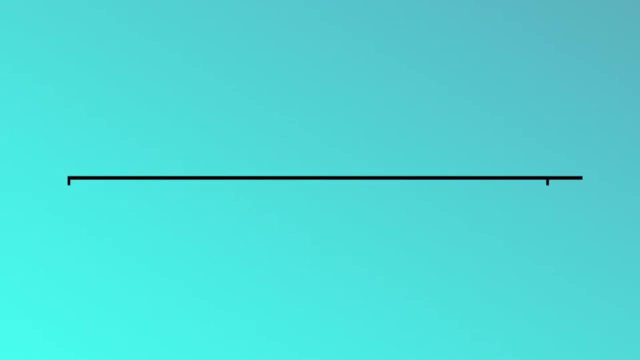 Okay, so back to number lines. Let's start by finding the fraction three quarters on a number line. The starting point of our number line is 0 and the ending point is 1.. This 1 refers to one whole. Now think about three quarters. 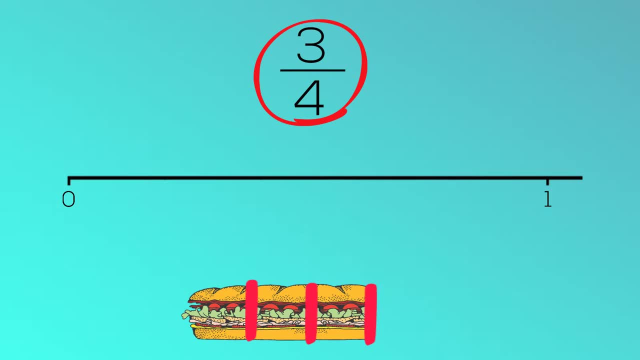 We know that three quarters is less than one whole. That means the fraction must go somewhere between the 0 and the 1.. Looking at the denominator, we can see that the whole has been split into four equal parts. Just like the sandwich, we need to split the whole represented on this number line into four equal parts. 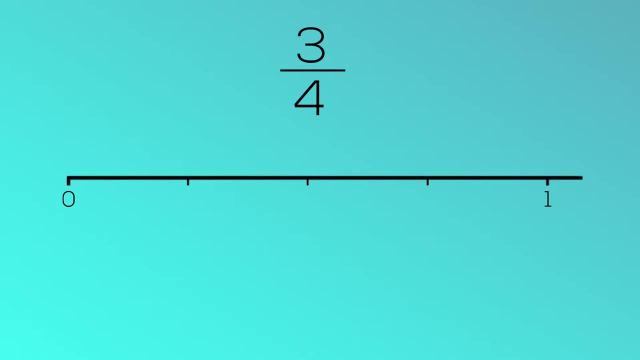 Now we need to look to the numerator to work out how many fourths we have divided into four equal parts, To work out how many fourths or quarters we have. we have three. Let's count along: One quarter, two quarters, three quarters. 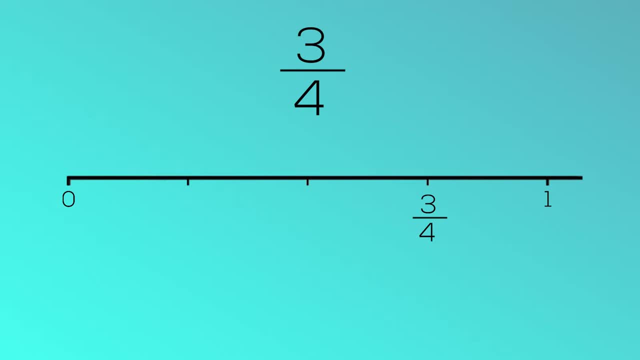 We have found the fraction three quarters on this number line. Here's another fraction for us to find on a number line: Two fifths. Here's our number line. We know that two fifths is less than one, so let's go ahead and fill in our start point 0, and our end point 1.. 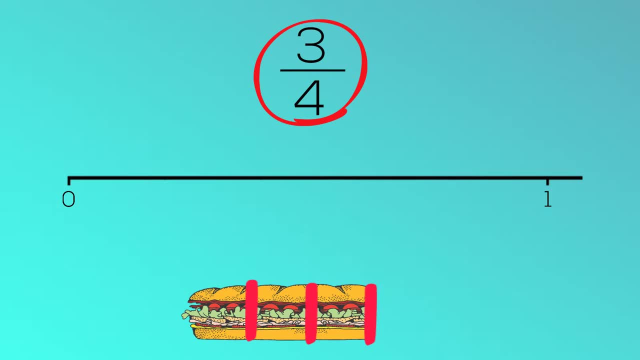 We know that three quarters is less than one whole. That means the fraction must go somewhere between the 0 and the 1.. Looking at the denominator, we can see that the whole has been split into four equal parts. Just like the sandwich, we need to split the whole represented on this number line into four equal parts. 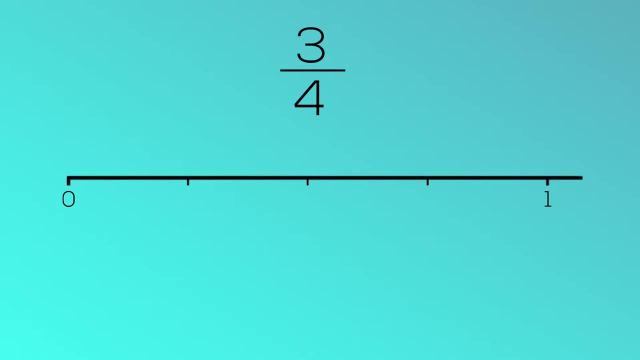 Now we need to look to the numerator to work out how many fourths we have divided into four equal parts, To work out how many fourths or quarters we have. we have three. Let's count along: One quarter, two quarters, three quarters. 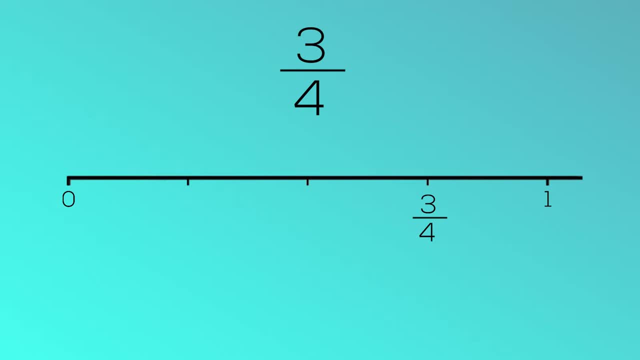 We have found the fraction three quarters on this number line. Here's another fraction for us to find on a number line: Two fifths. Here's our number line. We know that two fifths is less than one, so let's go ahead and fill in our start point 0, and our end point 1.. 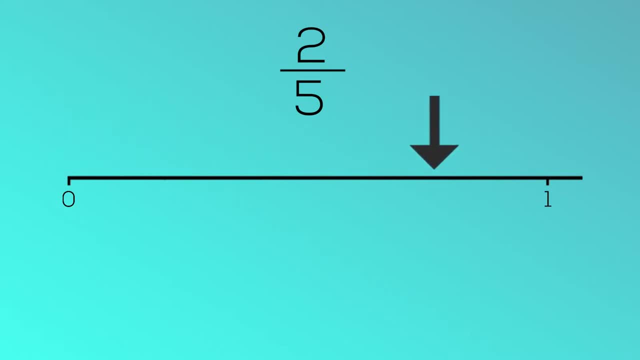 From the start point to the end point of our number line is one whole. The denominator is 5,, which tells us that the whole has been split into five equal parts. Let's divide the whole on our number line into five equal parts, We have found that two fifths is less than one. so let's go ahead and fill in our start point 1.. 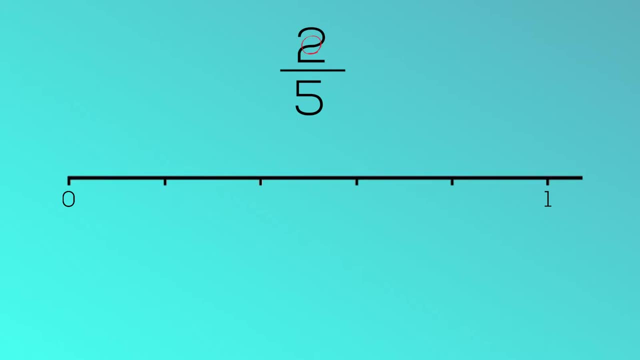 From the start point to the end point of our number line, we have two fifths. Now our numerator tells us that we have two fifths. Let's count along One fifth, two fifths. We have found two fifths on the number line. 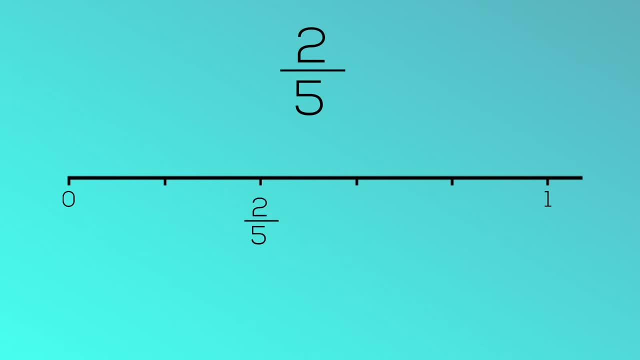 Here is another example. Here we have a number line and a marker. The marker is between 0 and 1, so it can't be a whole number, It must be a fraction. Let's work out how many fourths we have divided into four equal parts. 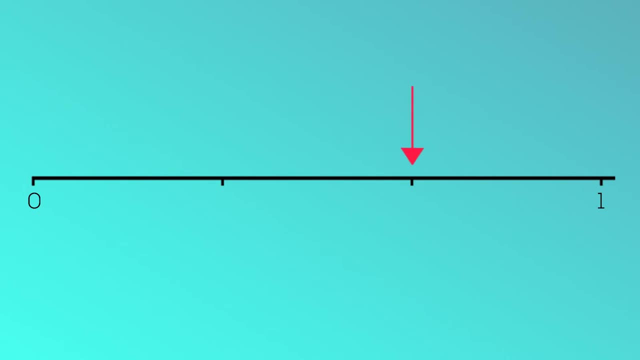 Here's another example. Here we have a number line and a marker. The marker is between 0 and 1, so it can't be a whole number, It must be a fraction. Let's work out what fraction belongs here. Let's work out what fraction belongs here. 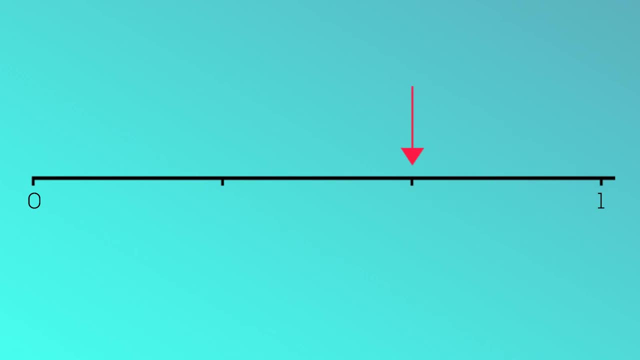 One whole has been divided equally into three equal parts. One whole has been divided equally into three equal parts. So each of these parts represents one third. So each of these parts represents one third. So each of these parts represents one third. One third, two thirds.